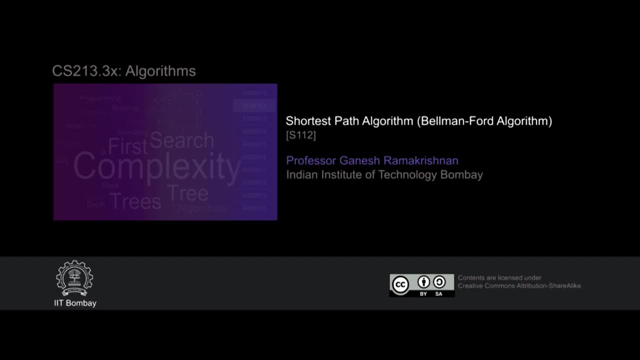 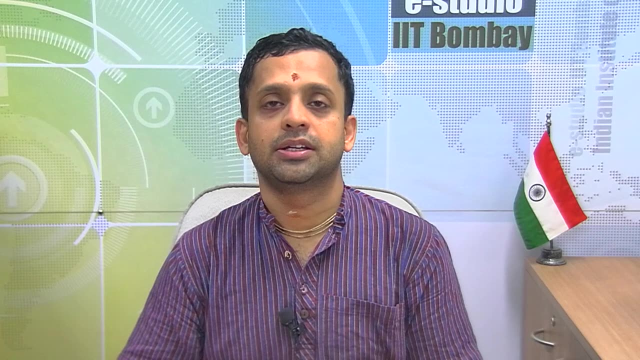 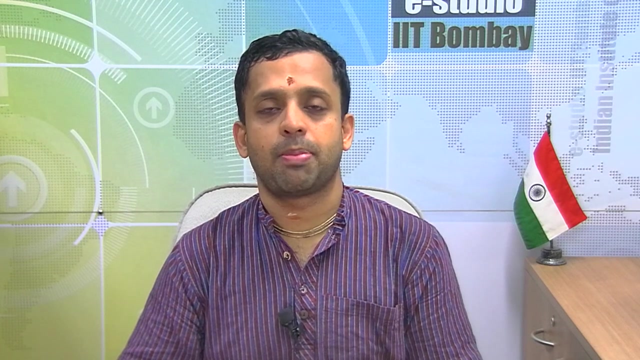 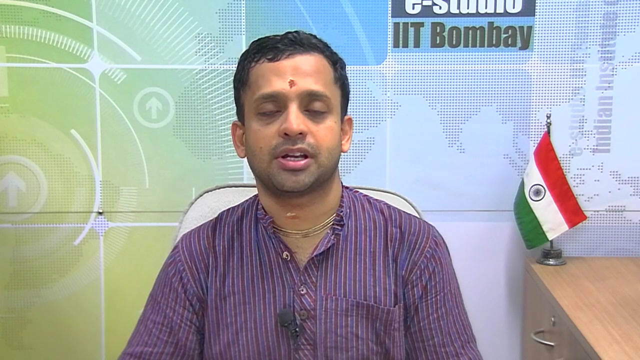 Hi and welcome to this next lecture on data structures and algorithms. We will continue our discussion on shortest path algorithms. In fact, we will continue our discussion for shortest path with a fixed source. However, today we will discuss an algorithm that can deal with negative weighted edges. Recall that we discussed Dijkstra's algorithm, which 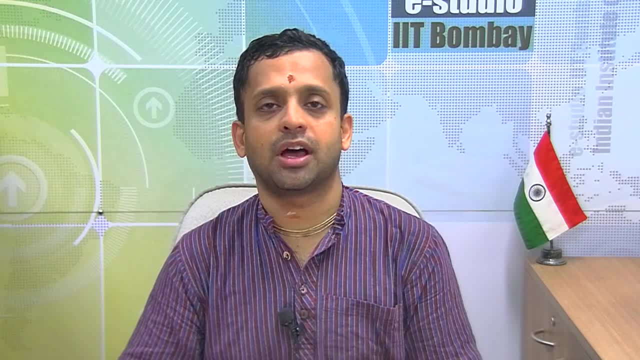 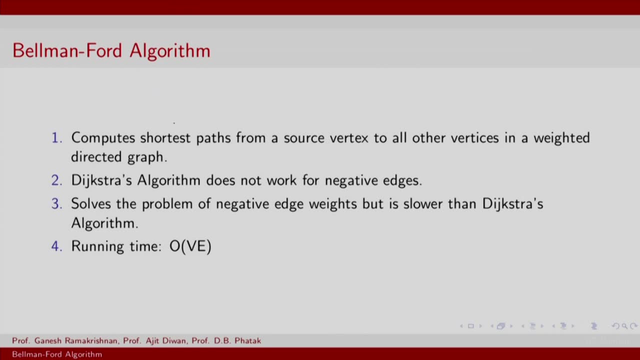 operates under the constraint that no edge weights are negative. So the Bellman-Ford algorithm. it computes shortest paths from a single source, fixed source, to all other vertices in a weighted directed graph. However, Dijkstra's algorithm does not work for negative. 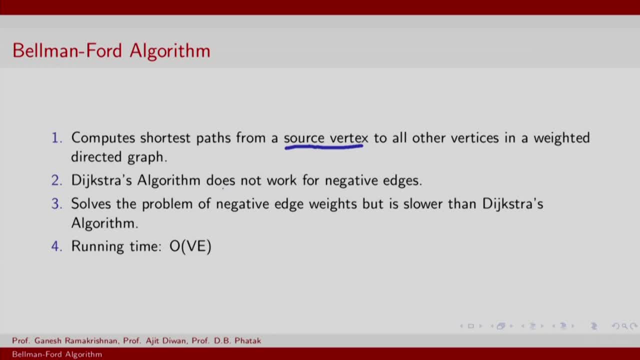 weighted edges. It is a greedy algorithm that makes use of the optimal substructure property. Bellman-Ford solves the problem of negative weighted edges, but it is slower than Dijkstra's algorithm. that is the price being paid And the running time is. 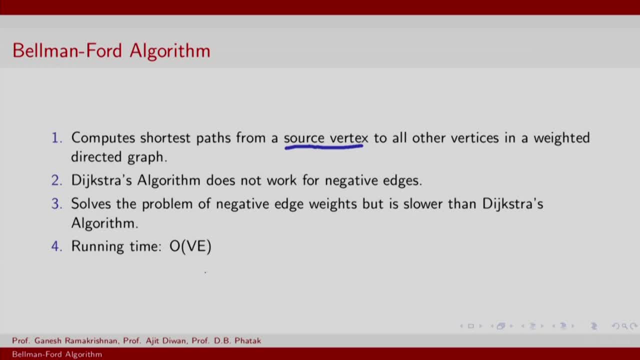 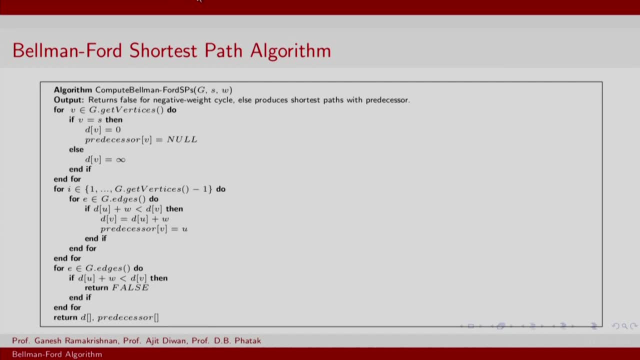 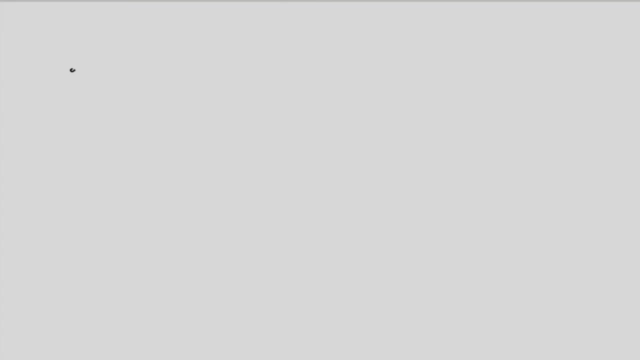 order of number of vertices is to the number of edges. So what is the idea? So let us understand the algorithm with a simple example. So we will try and illustrate the working of the Bellman-Ford algorithm through an example. 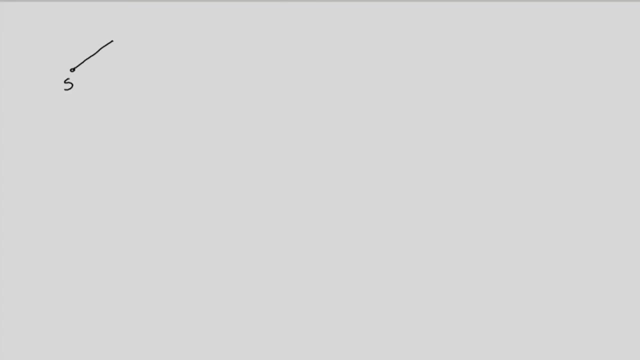 So let us say, your graph with a source is, we will consider a purely directed graph. Let us give names to these vertices: v1, v2, v3, v4, v5 and v6.. We will also give names. 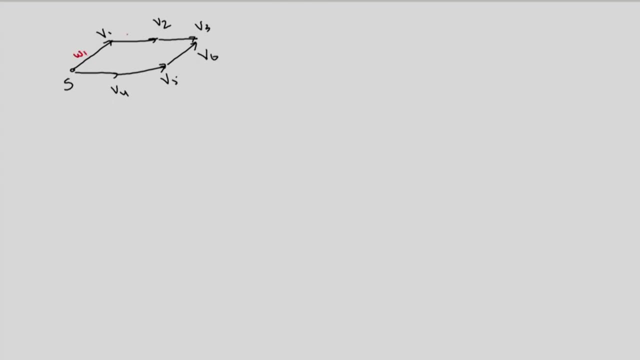 to the edges and their weights: w1, w2, w3, w4, w5, w6.. It also helps to have an additional edge here to make the graph a directed acyclic graph. So let us say this is w7.. 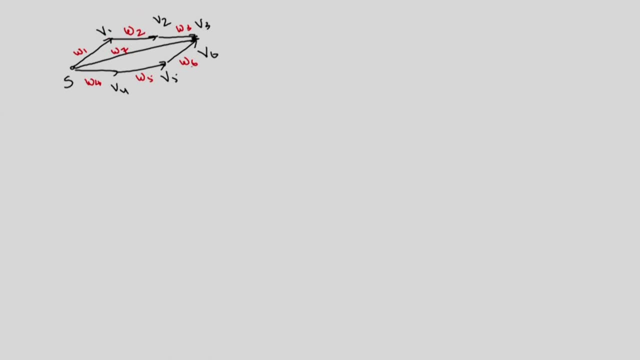 So Bellman-Ford algorithm iterates through all the edges of the graph. So the value of the edge here is the length, the length of the graph, the length of the graph- And for every edge it determines the weight on the two nodes that it is part of. 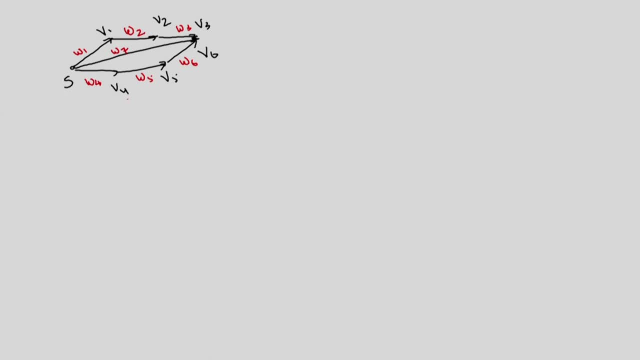 So, of course, if you have the edges to be undirected, it is possible that the shortest path crosses that particular edge in either way, in either direction. However, the edge is directed and half-directed. It can be very simple, because both are directly fixed. The 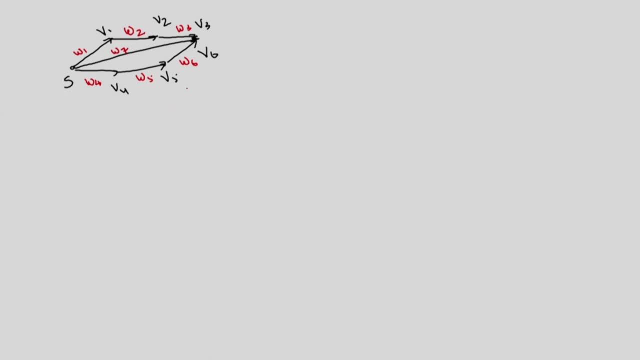 You expect the shortest path from one node to other node, if at all, to occur only along the direction that is permitted by the edge. So the idea behind Bellman-Ford algorithm is: initially, all vertices are infinitely far away from the source. The source is, of course, 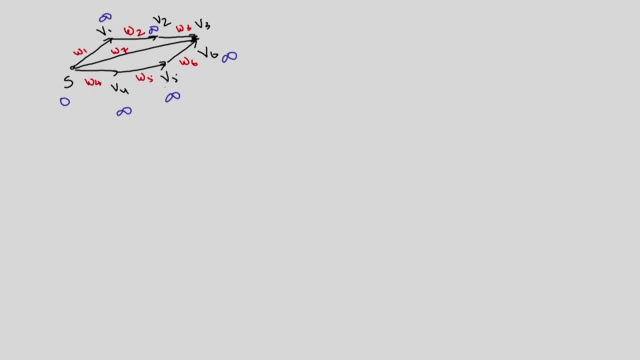 a distance 0 from itself. Now you iterate over all edges. for each edge, You are going to check if, let us say, e is going from u to v. You will check if the distance- the shortest path distance to v- existing distance, is greater than equal to the distance. 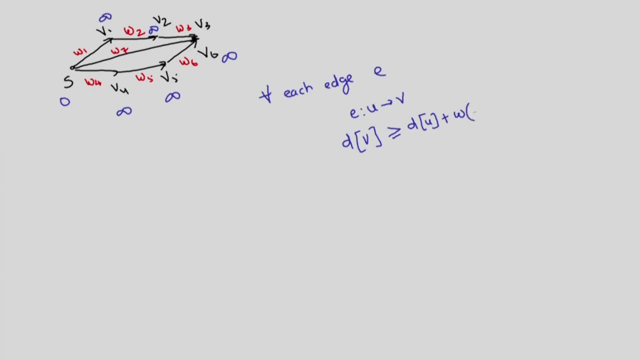 to u plus the weight on the edge u v. So this is the distance that you are going to get. If this is the case, then you update dv to this new found shortest path. It says I am going to look at the shortest path to u and then append the edge u v to the shortest. 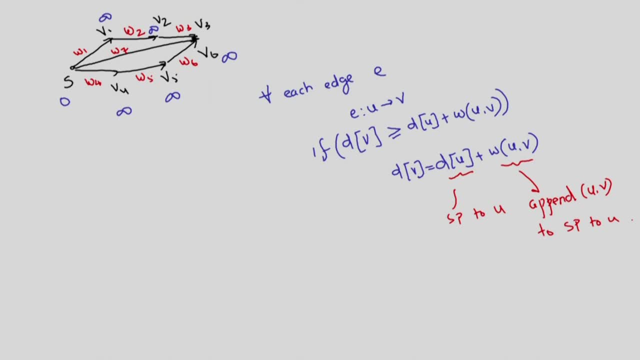 path to u. So this is the basic idea, And you are going to do this with every edge. How many times you will have to do? Well, when you start the iterations, initially you determine that for v1 and v4, or that is the 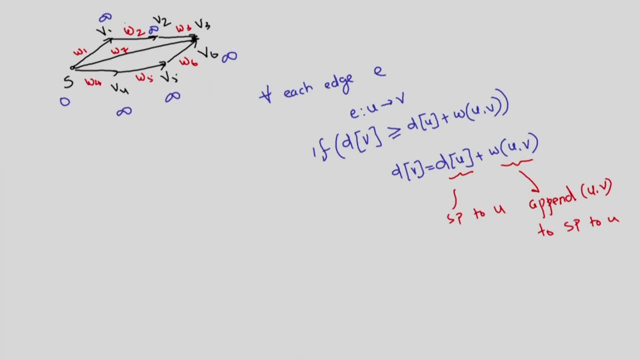 edges w1 and w4, you are able to update the weights for v1 and v4 to say w1 and w4 respectively. However, for all the other vertices other than source, of course, in the first iteration over all the edges there is nothing to update. However, in a subsequent iteration you will. 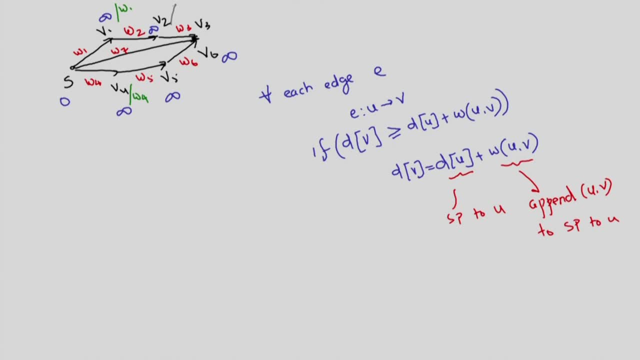 also update the shortest path for v2, say, which is w1 plus w2, and that for v5, which is w4 plus w5. So you will have to iterate over all the edges number of times. that equals the maximum number of hops to a node from S. So number of times to iterate over all. 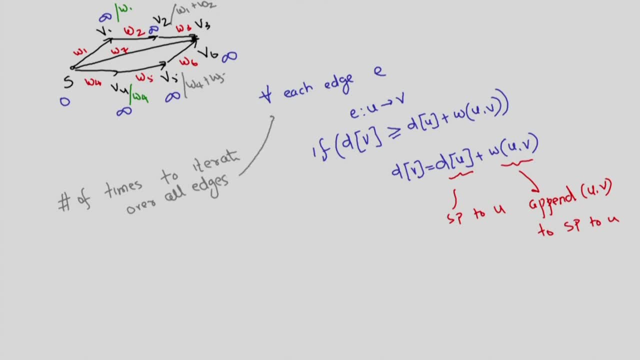 the edges. what I mean by this? This is this iteration, this is the width of graph, which is max number of hops from source node S to any vertex. say this: let us say v, v2,, v3,, v4,, v5,, v6,, v7,, v8,, v9,. 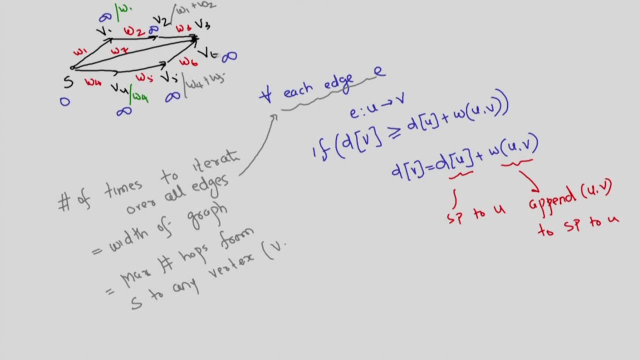 v10.. By the way, we do not need the v6. So I am just going to v3.. So this is going to be v3.. So the complexity is basically number of edges into this maximum number of hops. 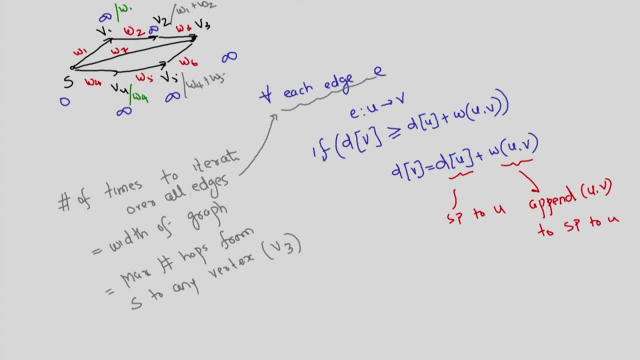 But I will convince you that this maximum number of hops, the worst case, actually happens to be number of vertices minus 1.. I will construct an example to show this. So let us consider a simple linear graph: S goes to v1, goes to v2, goes to v3.. So my first scan over the edges I will be able to. 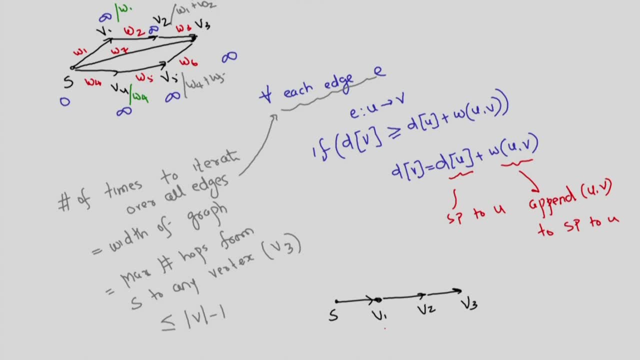 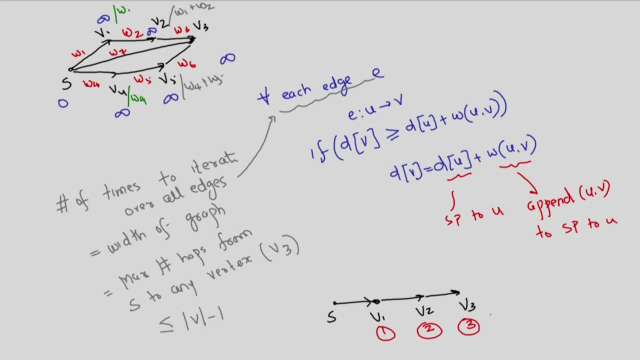 update v1, the second scan, I will be able to update v2, the third will be v3.. So there are four vertices and I need three verticesビ. 3.In the circuit, I need three vectors to be able to update v1 and the third to be able to update v2.. So I will construct an example. 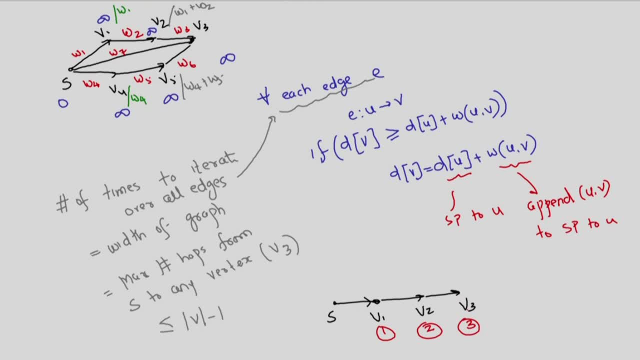 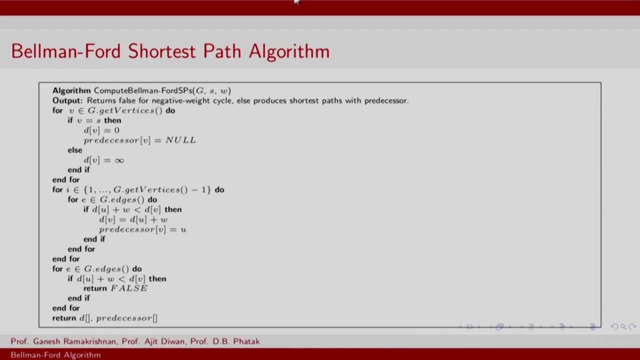 and I need 3 scans over all the edges till I am able to reach V3 and update its shortest path. I can update the shortest path for V3 when the shortest path for its immediate neighbors are updated. Let us look at the actual algorithm. As pointed out, the first thing you do is: 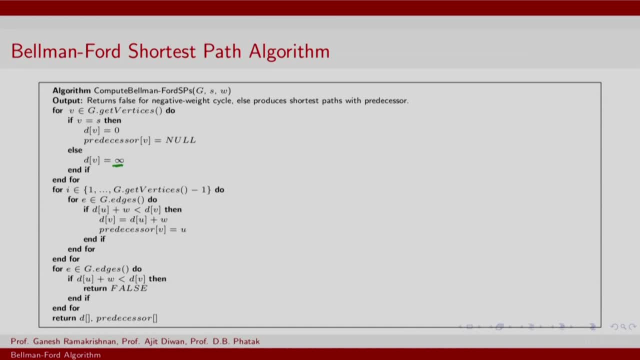 iterate over all the vertices, set the depth of every vertex, the shortest path to depth, to infinity. The predecessor for all the nodes is not set, but the predecessor for the source is null and the depth for the source is 0.. And then, as suggested, we are going to iterate. 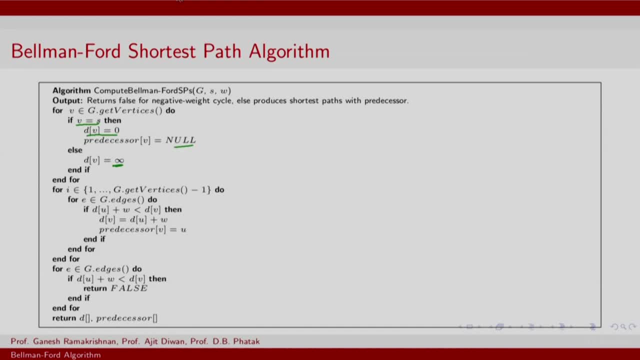 over all the edges. this inner loop iterate over all the edges, and we are going to do that for a number of times. that equals number of vertices minus 1.. So recall that we have requested the��ing. Let us see how we can do it. Let us try it. So see this: this is the площad, So it is. 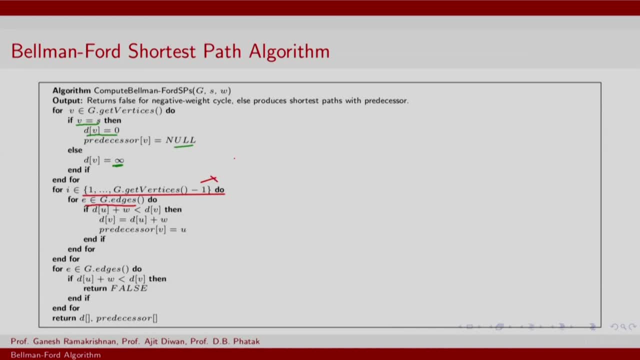 the electrode which gets first finely interested at the point V of its longitudality and then at the point s. So suppose we need to donut and thatетрide, because if both of them do not conform GDP local, this is the bottom itizar at the point Ft1.. So here you take. 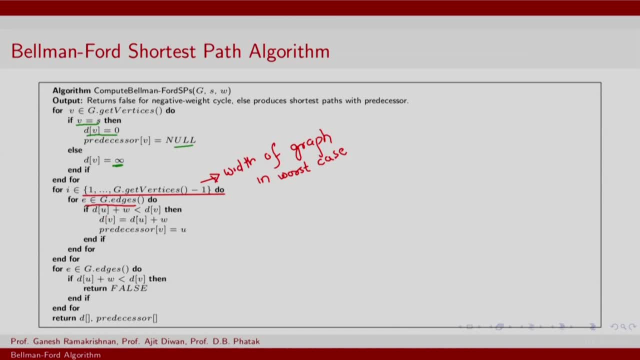 du plus w. w is the weight of edge e. If this happens to be less than the existing shortest path distance to v, then you update the shortest path distance at v. You also update the predecessor of v to point to u. So this is already motivated and explained. What is the part here? at the 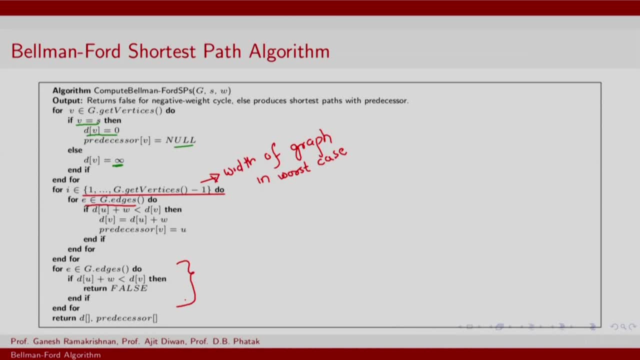 end. Well, so far, we have assumed that our graph is a directed acyclic graph. What if the graph has cycles and is therefore not a directed acyclic graph, abbreviated as DAX data? Even in the case that the graph has no directed edges, it might just have cycles. 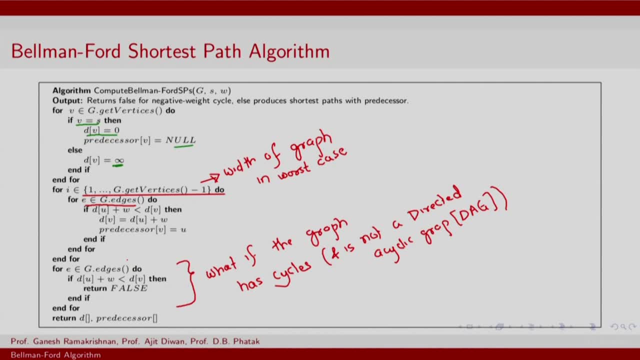 And here is a test: If the shortest path can be further reduced, even after v minus 1 iterations, then it appears that there is a cycle, That is, there is a path from s to v. So this is a path from s to a node, any particular node that involves a cycle. 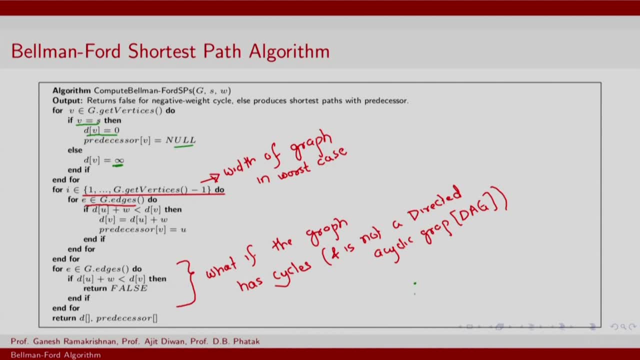 Let us illustrate this with an example. So we have s v1,, let us say this is weight 5. This is say 4 to v2, v3, minus 3.. We already pointed out the negative weighted edges are: 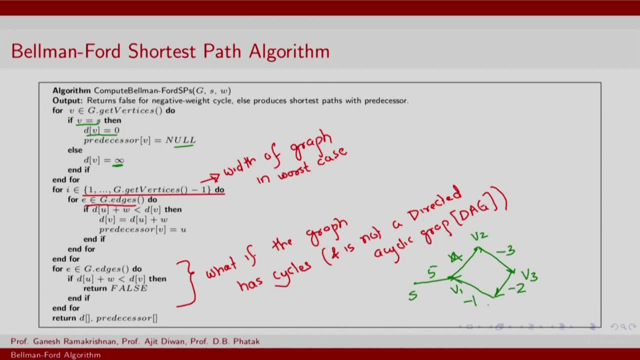 0 and say minus 2, minus 1.. Now, as you update the weights originating with s, 0, v1 is 5, v2 is 9, v3 is 6, and then you have 4, and then you have minus 1,, 3,, minus 2, and then you have. 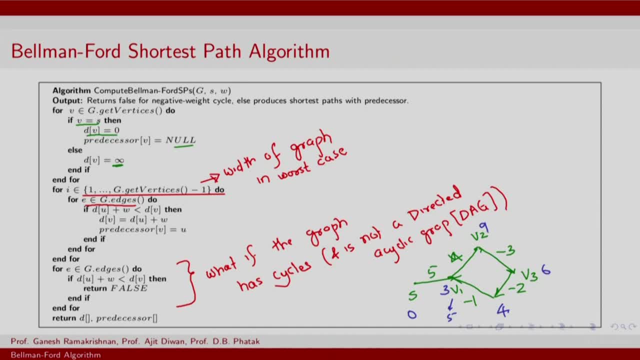 0. So that is the one you have, and then you have minus 1, v2 is 5, v3 is 6, and then you have, However, the next iteration. when you update V2, you will get 7, and then you will be able. 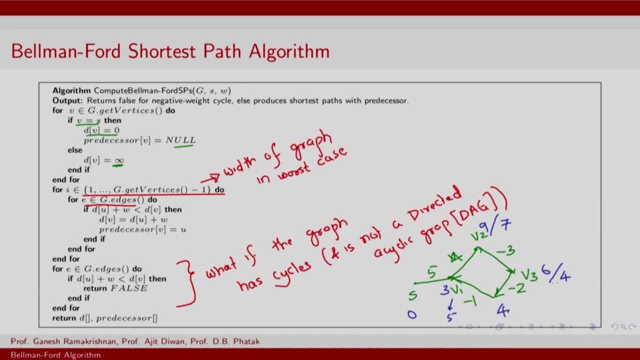 to update V3 to 4 and that at this node, V4, you are able to update the weight for V4 further and get it to 2 and then at V1, get it to 1.. You could do this again. go over this. 1 plus 4 is 5, 5 minus 3 is 2,. 2 minus 2 is 0, 0. 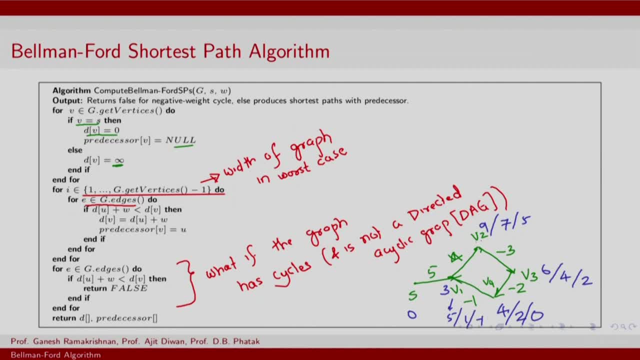 minus 1 is minus 1, and so on. So just by going around this loop you can actually get very, very negative weighted paths from S to all of these nodes. So what is the characteristic here? Well, it turns out that this cycle itself has negative 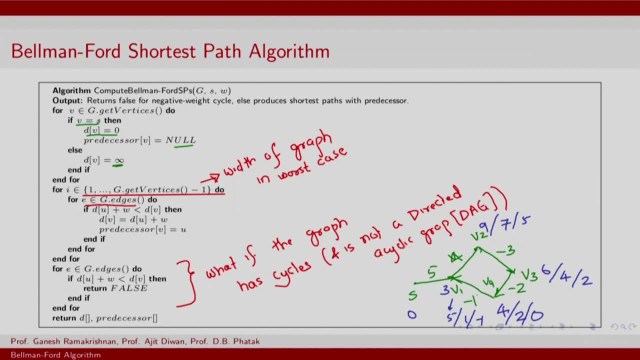 weight. What is the weight of the node Of all paths on the cycle? minus 1 plus 4, plus minus 3 plus minus 2, the whole weight is basically minus 2.. So the more you go around in this loop, the more you will be able to reduce the shortest. 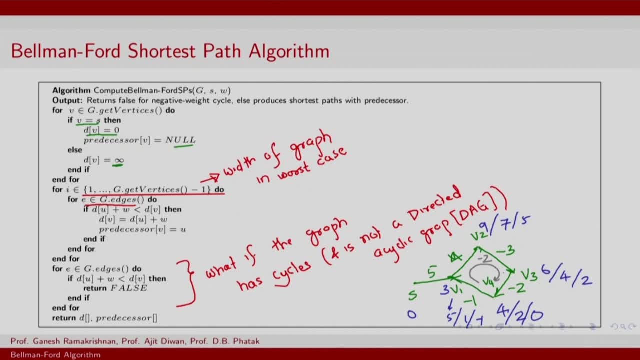 path, and this you can do ad infinitum. So this is what we are checking: If, after so many iterations, if you are still able to reduce the shortest path distance to any particular node, then you basically cannot find a shortest path, So you just return a false. 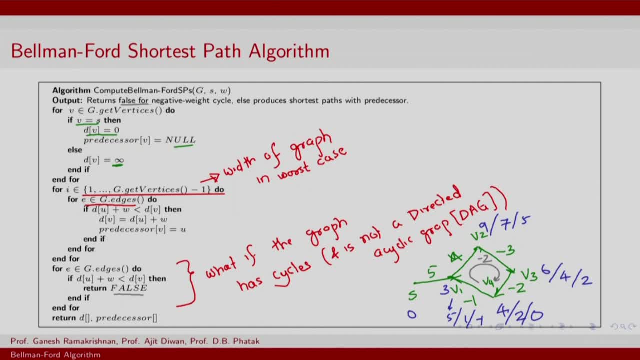 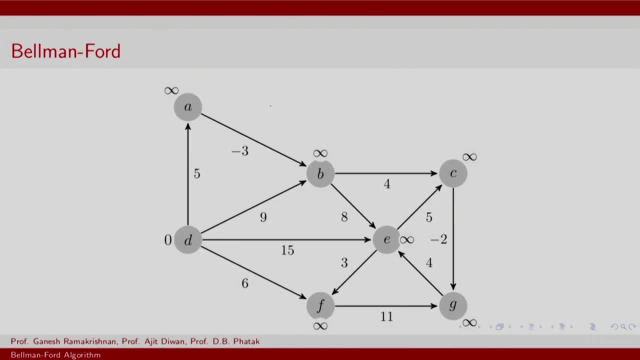 So that is what we see here- returns false for negative weight cycle. Let us see this in action. We start with infinite weighted shortest path to all the nodes, The first iteration, over all the edges. we find that only the immediate neighbors of the source can be updated, and we have done that. 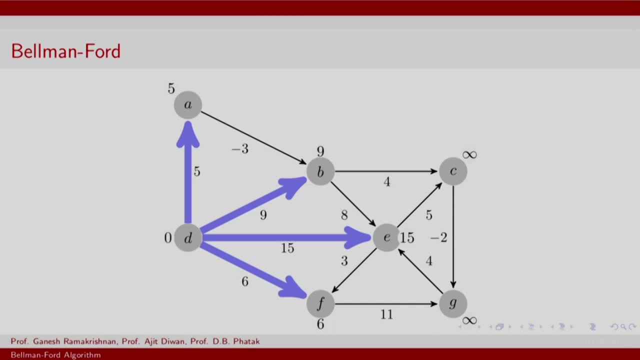 Then again we look at all the edges. we are only able to update now the immediate neighbors of these nodes that were updated. So it turns out that B is also neighbor to A and you are able to get shortest path to B through A. This is the latest. 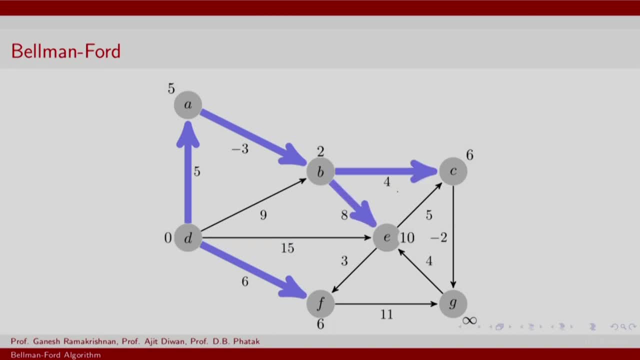 We continue our bookkeeping, Find that the shortest path to C and D has been updated, C and E has been updated, And then to G. Okay, And it turns out that you can actually find another shortest path- G, through C And in. 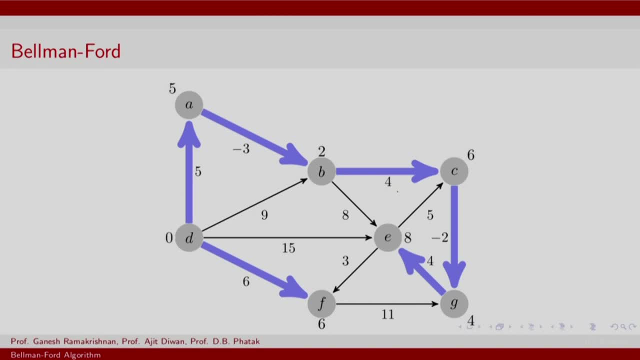 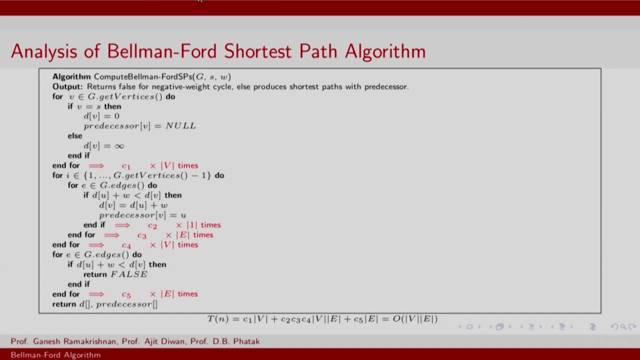 fact, this also lets you update shortest path to E through G. So let us analyze the Bellman shortest path algorithm. We look at two characteristics. One is its correctness and the other will be its complexity. So we prove the correctness of this. We are going to try to query S as well. 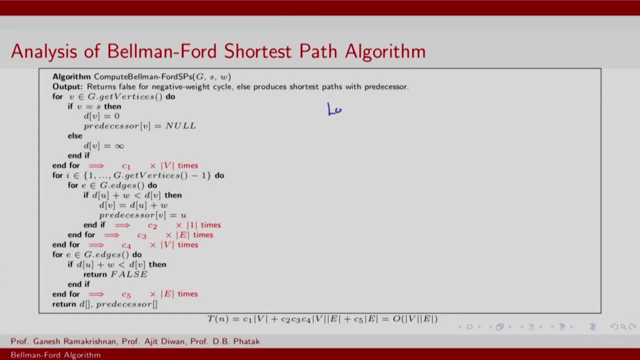 Now, this is a passiert, right. This is what is happening. this is what we are going to do. This is what is happening. We are going to query S as well. So what is happening in this case? The answer is: we can compare it with Thomas Hill's method of determining the original. 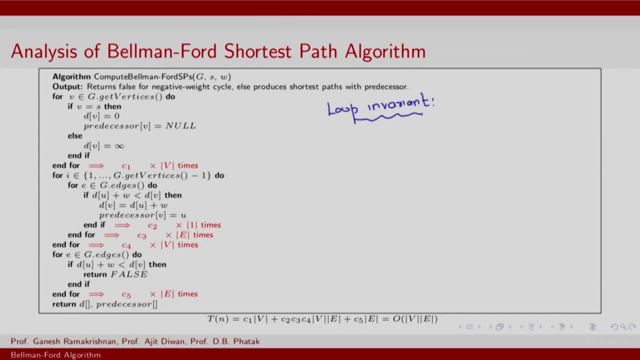 vertical axis, and the next instance we will go to is the little bit All right Now. if you look at this one over here, you will find that it goes up and down. If you look at this one over here, you will find that it goes up and down, just like the. 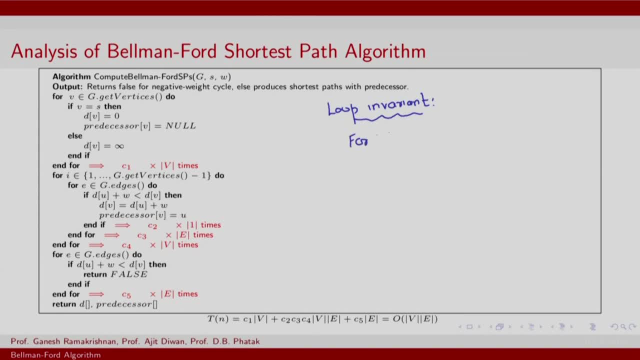 first step. okay, So this is the vertical axis and this is the horizontal axis. This is the vertical axis, So this will follow the horizontal axis, but the vertical axis has to be completely separated from the horizontal axis. vertex v: within k hops from the source, node S. the value d v is indeed the shortest path. 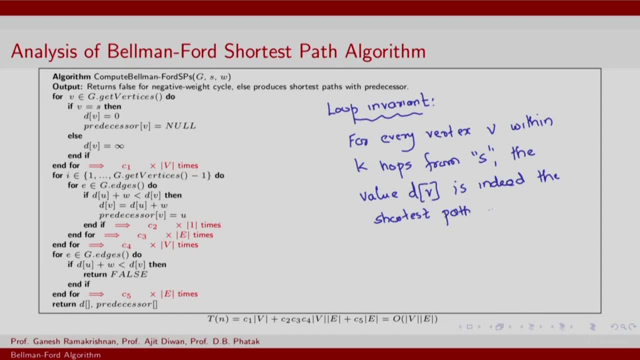 from S after k outer iterations. So we are claiming that at the k? th iteration the value that gets updated from the source node S is always the shortest path from the source node in dv. at the end of this kth iteration, dv contain the correct value: the shortest path. 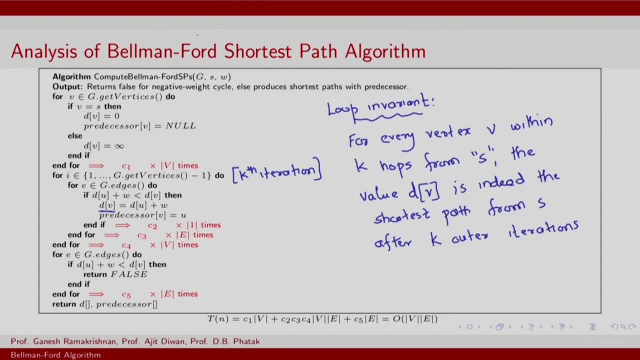 And it is easy to show that at initialization this is correct because the only node that is within 0 hops from the source itself, and indeed the depth of shortest path of source is set to 0.. The next iteration: we can easily see that we only deal with the immediate neighbors. 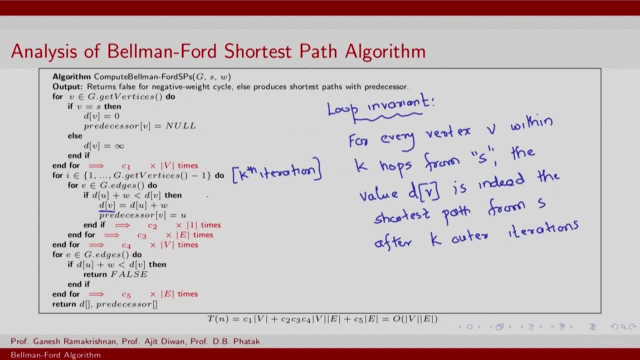 of the source and they get updated correctly. In fact, the maintenance can be easily proved because we know that to get to a vertex which is k plus 1 hops from the source S, you need to go through a vertex which is within k hops from the source S. 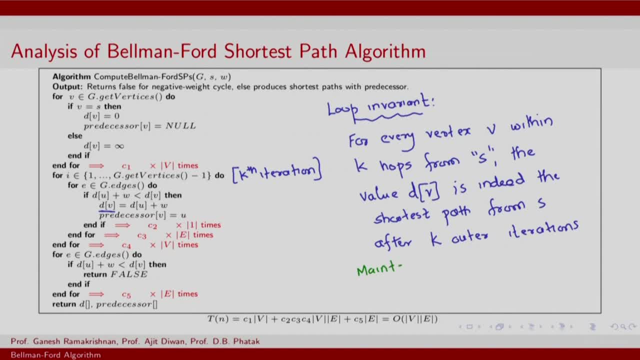 So maintenance, So maintenance. So maintenance can be proved with the key observation that a vertex at k plus 1 hops from S is reached through vertex at k hops from S, And this can therefore extend even at termination. What about time complexity? Well, the run time complexity is again straight forward.